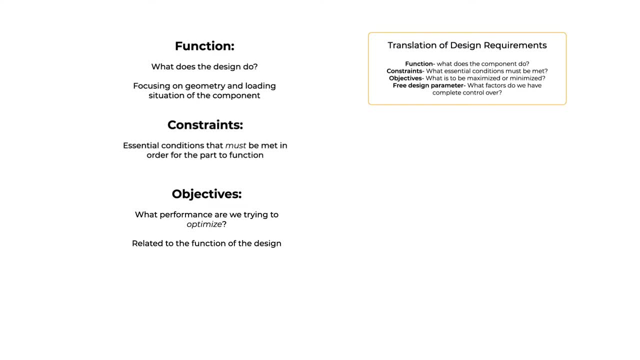 These are related to the function of the design, especially in the load-bearing component cases. And finally, we have the free design parameter. Since all materials are different, if we truly want to choose between them all equally, we need to have some amount of flexibility in our design. 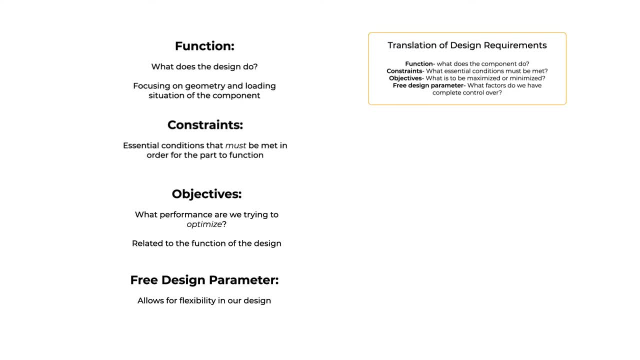 The free design parameter means that if we want to choose between them all equally, we need to have some amount of flexibility in our design. The free design parameter allows us to specify one aspect of our part, say the geometry, which we can change as needed. 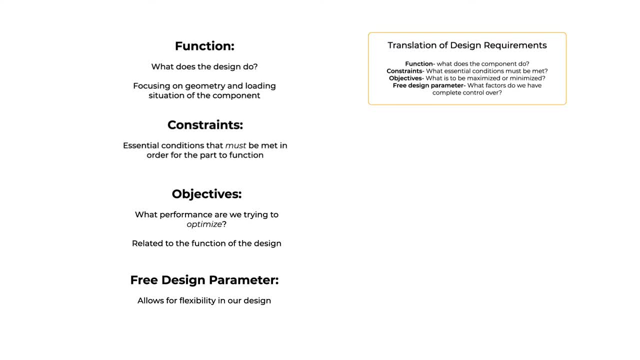 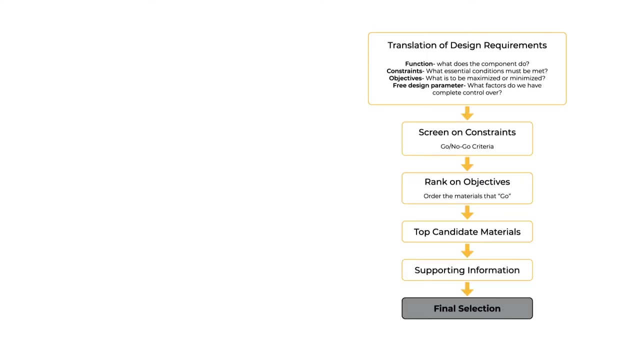 For example, flexibility in cross-sectional area allows us to choose between materials with different stiffness but achieve the same performance. Once we have our material properties and loading conditions, we can move on to our screening and ranking stages. If you watched our material selection using AshbyCharts Innovation Course, you're familiar. 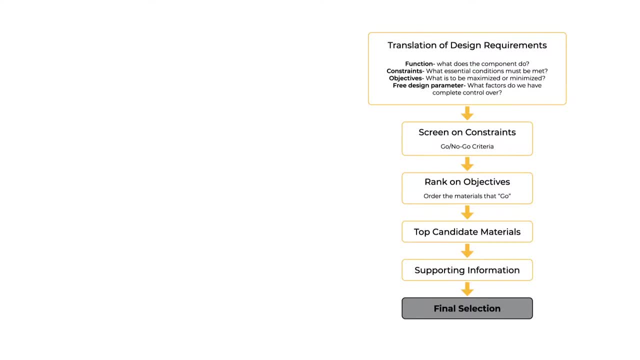 with these terms. First we scroll, First we screen our engineering materials based on the constraints. Constraints determine which material properties are acceptable or not for a design. Then we rank the materials that are left over based on our objectives, seeing which materials 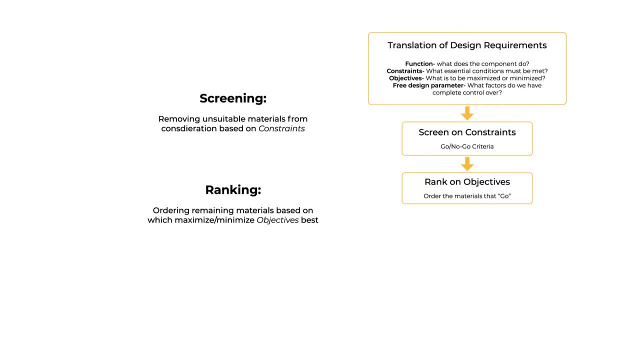 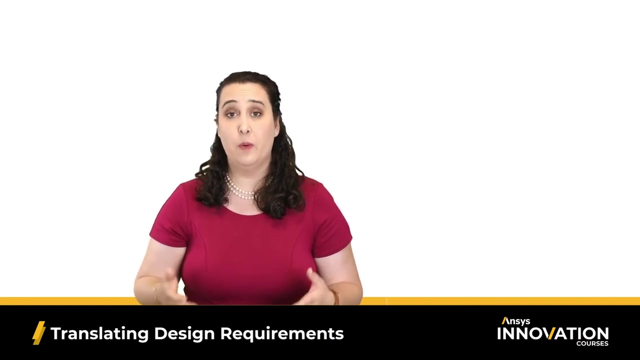 best maximize or minimize our properties of interest, their performance. After these steps, we're left with a few top candidate materials. At this point additional research is needed. We can see that we have a nice systematic way of going through our various design criteria. 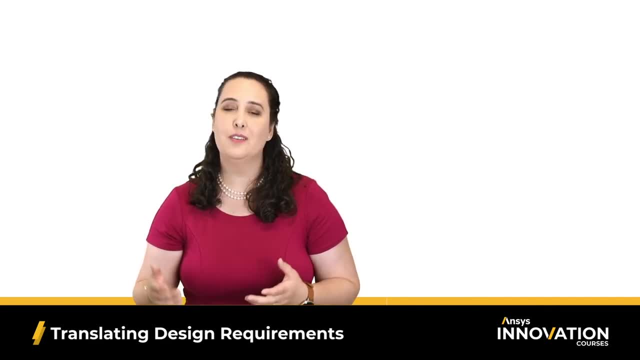 to get from thousands of engineering materials down to a few top candidates for our consideration. We can see that we have a nice systematic way of going through our various design criteria to get from thousands of engineering materials down to a few top candidates for our consideration. 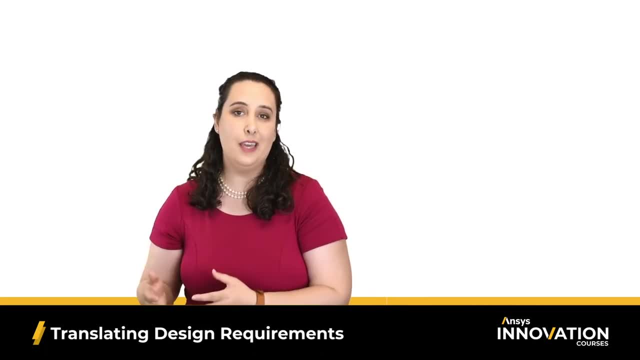 One tricky aspect of this methodology is the translation step: getting from our design problem statement into these key considerations. For example, if we were to do a new piece of research, we'd have to go to the same material and do the same thing over and over. 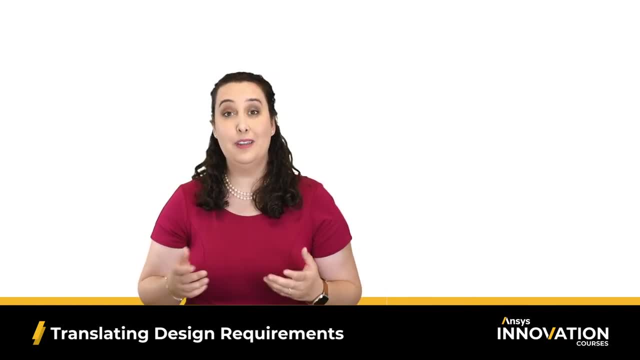 and objectives. So let's go through an example with a selection analogy. This is actually something I dealt with in my personal life. last year I needed a new car. It had been over ten years since I'd gotten my previous one and my life has. 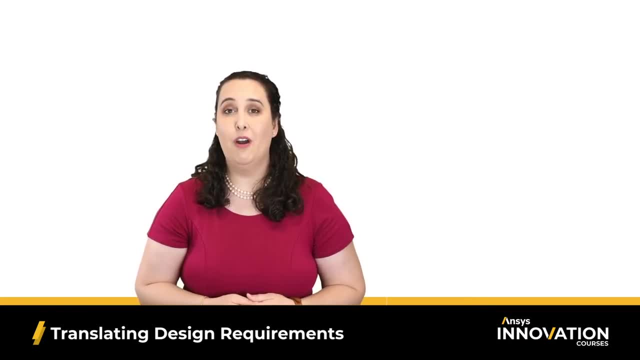 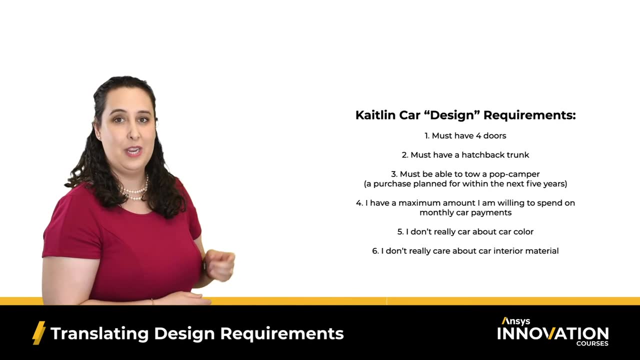 changed pretty significantly since, so my needs in my car have changed as well. So the first thing I did was write out a list of requirements, which I've shown here on the screen. My car needed to have four doors. Why? Because I wanted four. 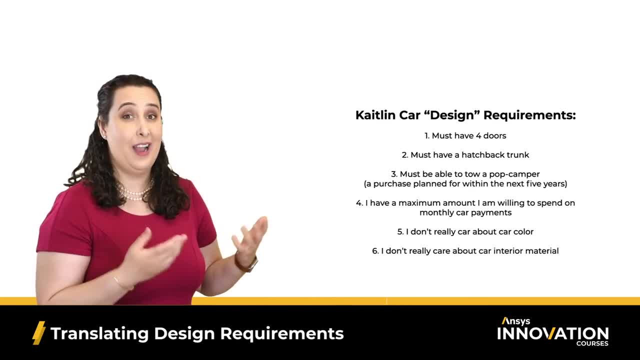 doors. Sometimes, when designing a product, your customer has some requirement that you need to meet, which may not have any technical merit, and that's okay. I also needed to have a hatchback trunk. I'm often carting various things around it. 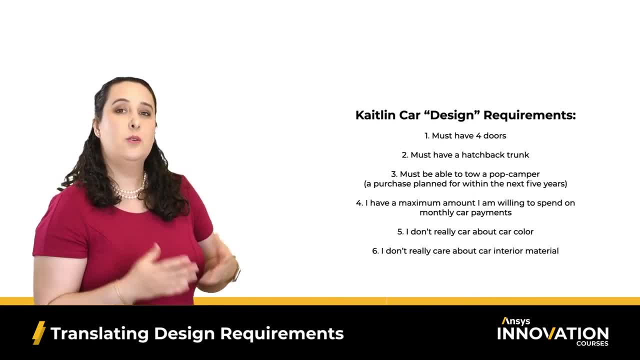 I need a place to put all my stuff. I also needed to be able to tow a pop-up camper. We don't own one yet, but my husband and I have been talking about purchasing one in the next five-ish years. I know I'll still have my 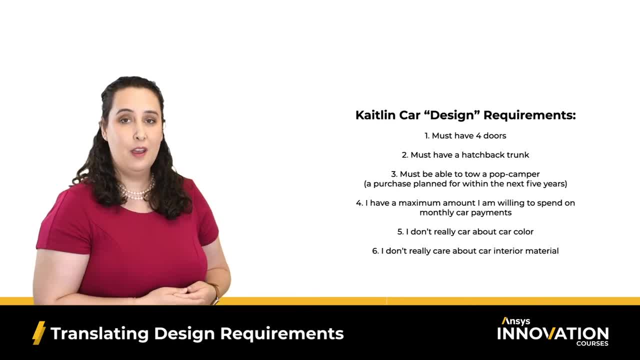 car at that point, so it needs to be able to tow it. I also had some maximum value that I was willing to spend for monthly car payments And, finally, I didn't really care about the car color or the material the interior was made out of. How do I? 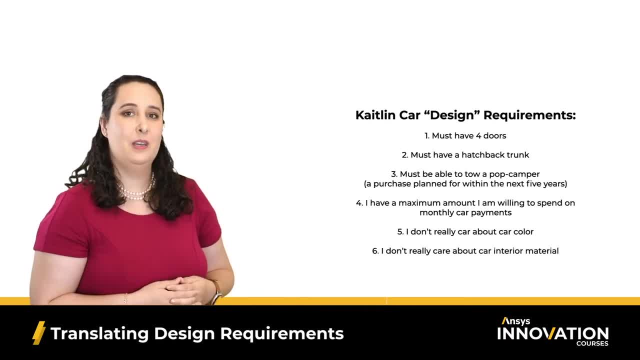 take this list and actually come up with a car. Well, I actually can use the Selection Methodology. It's easy to make a selection. I can select the car and I can make a selection. It's really easy to make a selection. I can actually make a selection, I can. 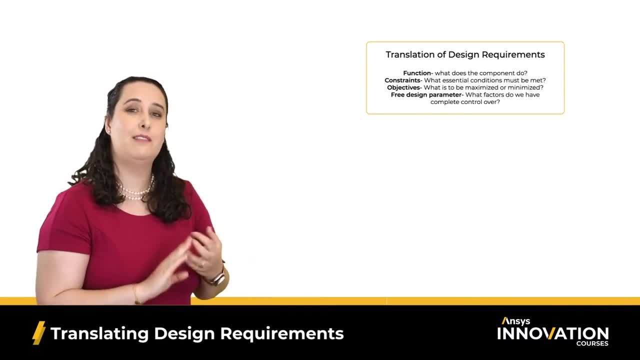 and break down these requirements into functions, constraints, objectives and free design parameters. So the function of my car is that it has to be able to transport me, my husband and our dog on various outdoor camping and hiking trips, as well as long-haul drives to see family and friends who live out of state. 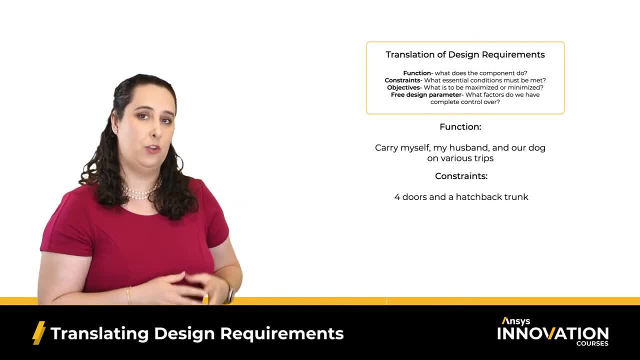 Our constraints must have four doors and that hatchback trunk. Now, why are these constraints? Well, if the car doesn't have them, I won't buy it. If we go back to when we were defining constraints, we said that they were our go-no-go criteria. 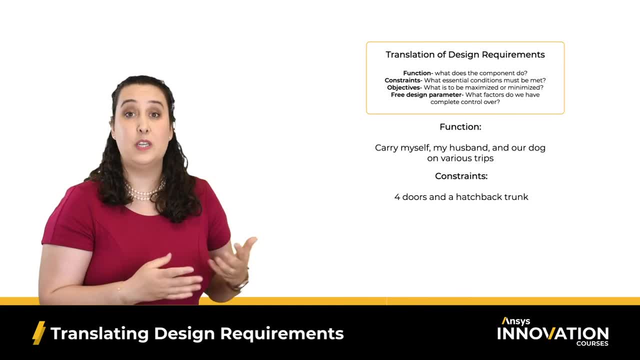 If the material wasn't able to perform in a certain way or didn't have specific properties, we needed to remove it from consideration. So any car that didn't have four doors or a hatchback trunk was removed from the pool of cars I was willing to consider. 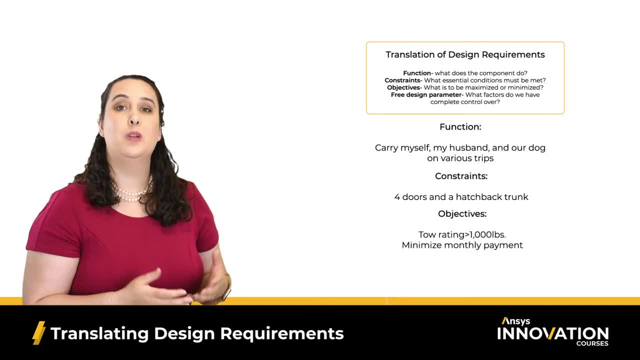 Next were my objectives. The first one was related to that tow rating. Now, we were also researching pop-up campers at this time and saw that most of the ones that we liked started at around 1,000 pounds. So I actually want to maximize the tow rating for my car.